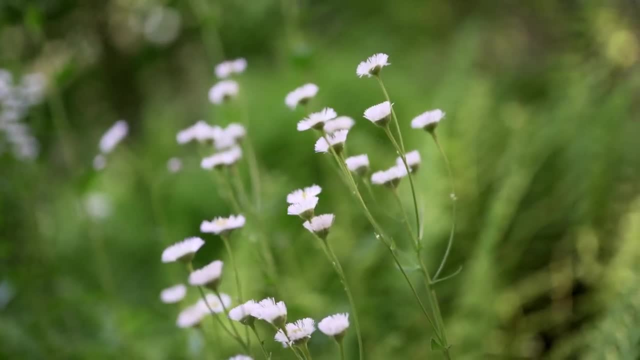 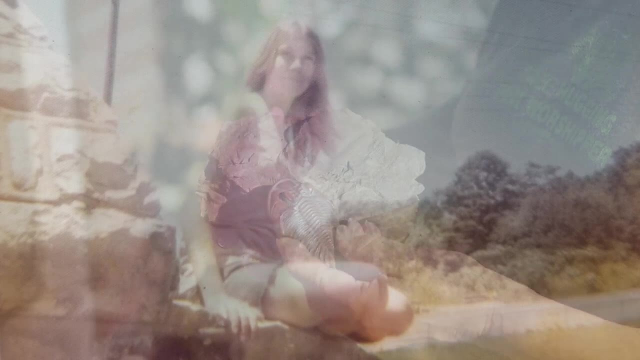 So I never really paid much attention to what she was searching for. I remember when she first found a trilobite and showed it to me, She was explaining why the find was so fascinating and the age of the creature All I could think about was the SETI eel from. 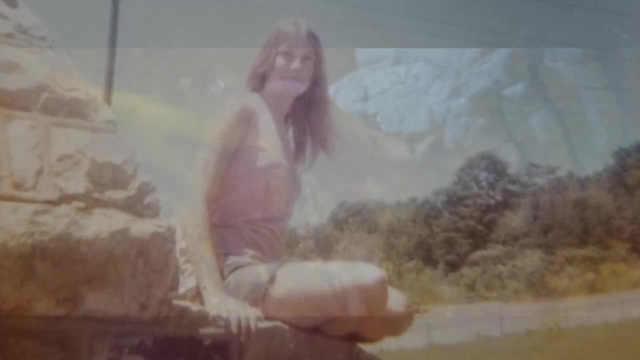 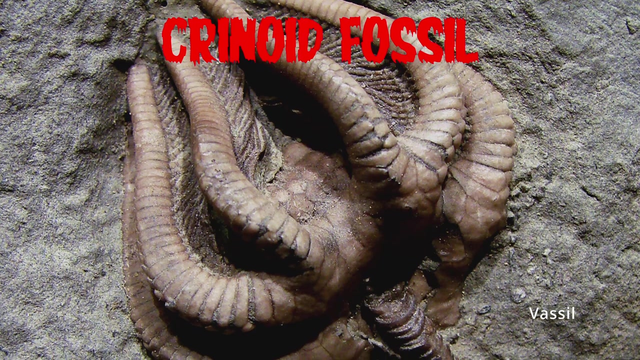 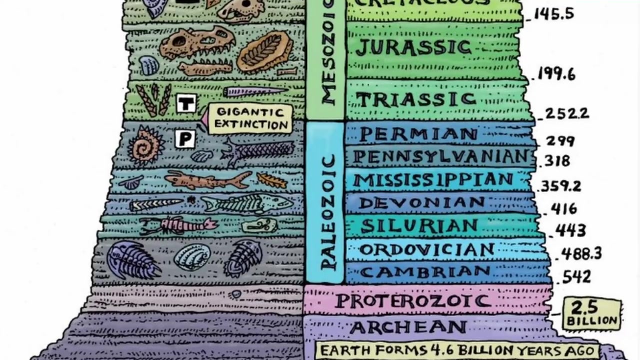 Star Trek II or the Rathacon and the facehugger from Alien. But it turns out that HR Giger's alien creatures were actually inspired by fossils from the same Paleozoic era as the trilobite. My mom explained that if you want to find a specific fossil then you have to search for. 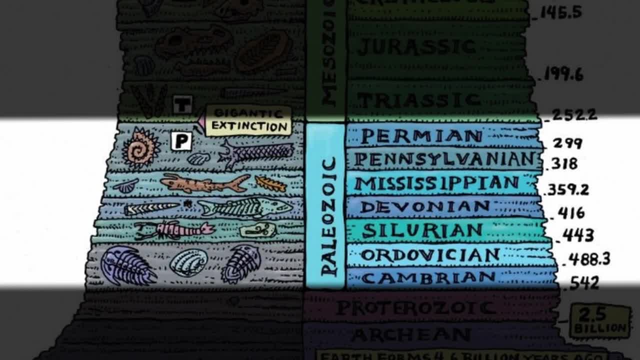 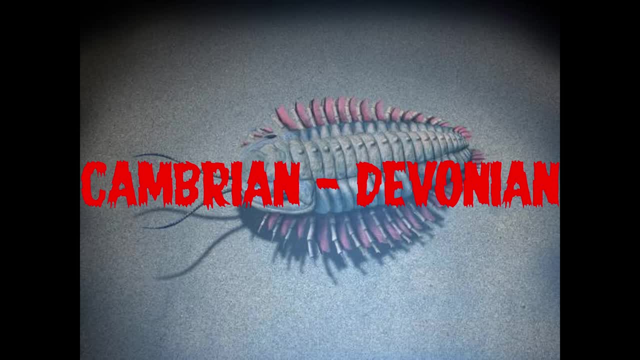 deposits that were left behind by specific errors of that creature's life. I wanted to find either a face-eating crinoid or a Star Trek mind-controlled trilobite. The trilobites began to decline during the Devonian period, so we headed towards that area of the state. 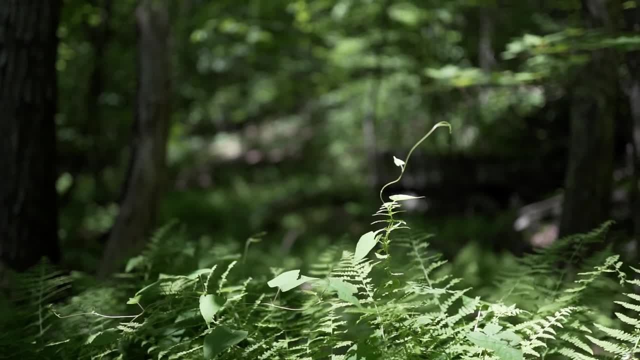 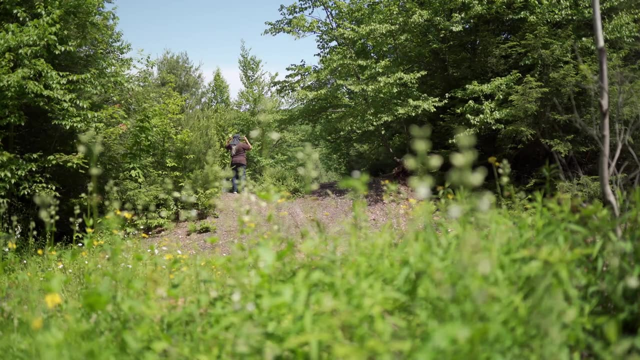 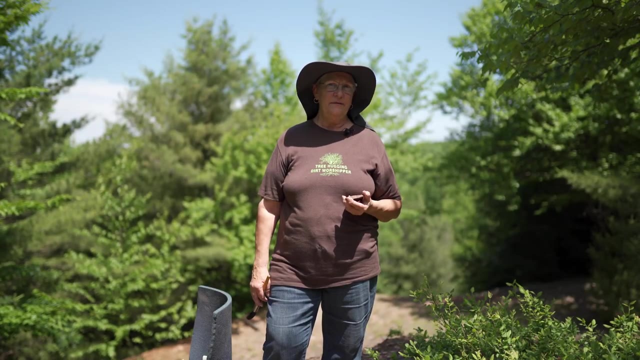 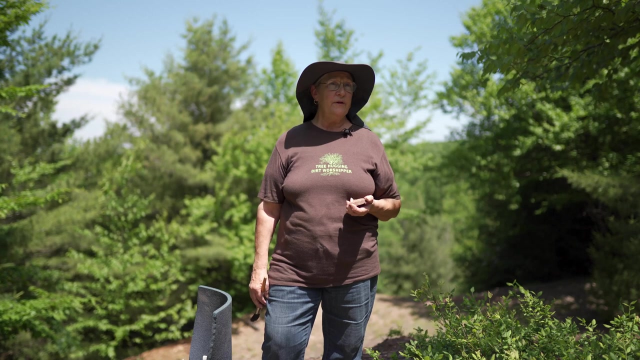 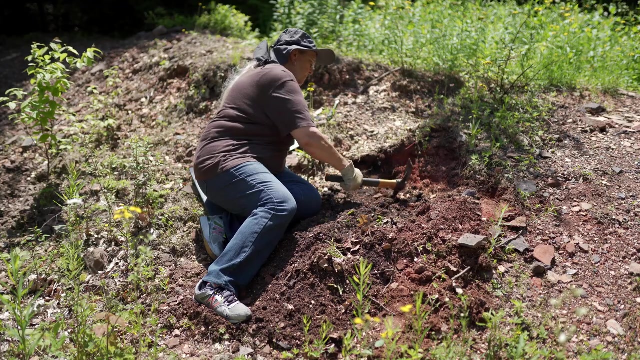 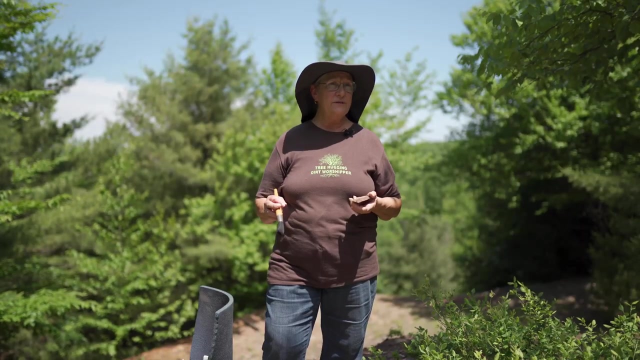 This was a forest back in the Devonian time and we're looking for fern fossils, tree bark, fossils from the Lipidodendron and even the roots of that tree. You can find fossils of that. You get a pick and you start digging through the mounds that are here. This area was these: 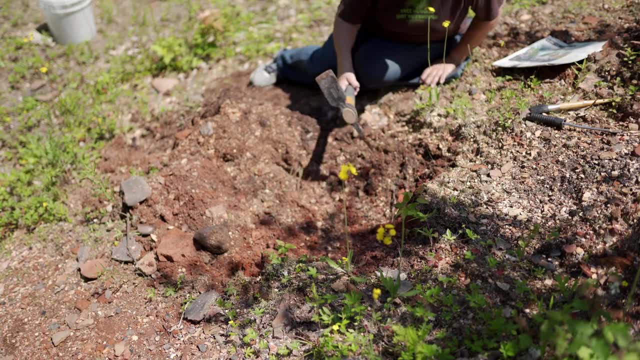 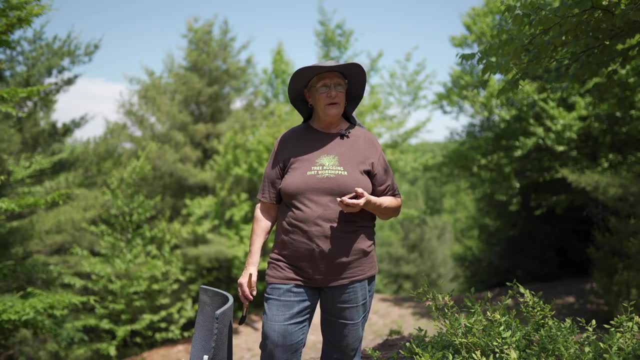 are coal spoils from a coal mining company. So we have a lot of things within those dirt mounds. so you want to get your pick out and you want to pick out the rocks and stones out of the mound and then carefully check them. I brush them off with this little brush. 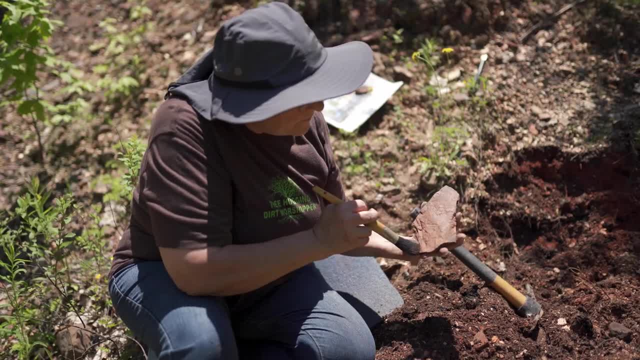 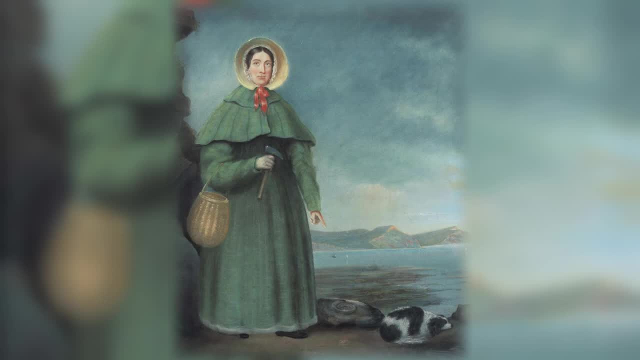 and you'll be able to see if you have a good impression. My mom follows in the footsteps of another female fossil hunter. Mary Anning was born in 1799 and became known around the world for the discoveries she made in Jurassic Marine fossil beds and the cliffs along the English. 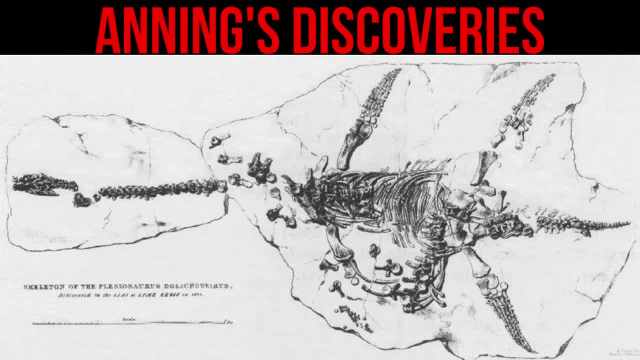 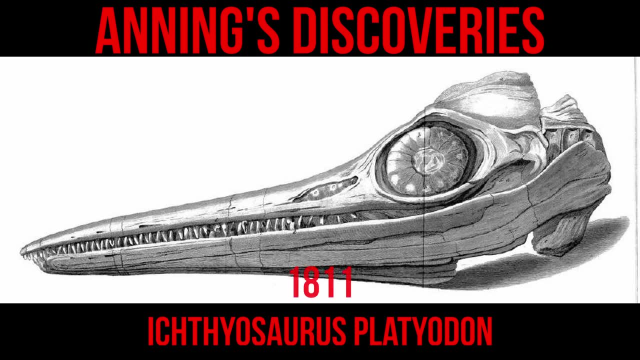 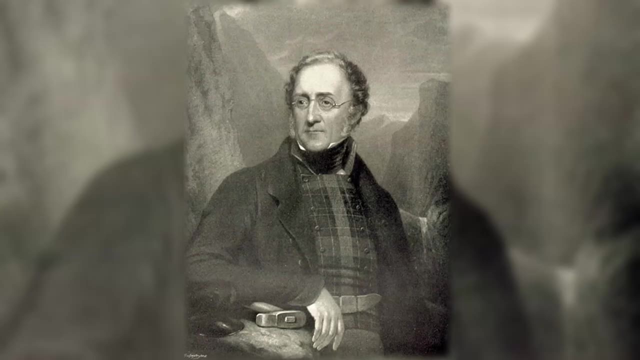 Channel in southwest England. As a woman she was not eligible to join the Geological Society of London and she did not always receive full credit for her scientific contributions. However, her friend geologist Henry de la Beck, who painted Duria Antiquor the first, 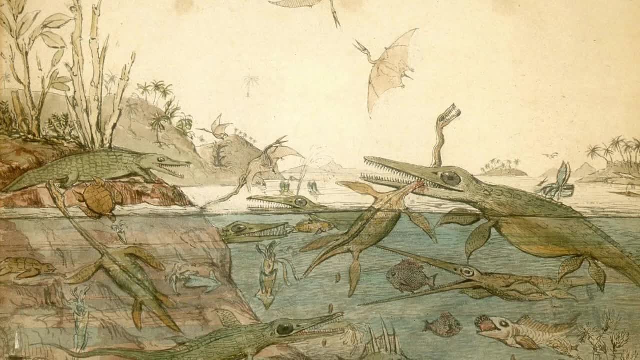 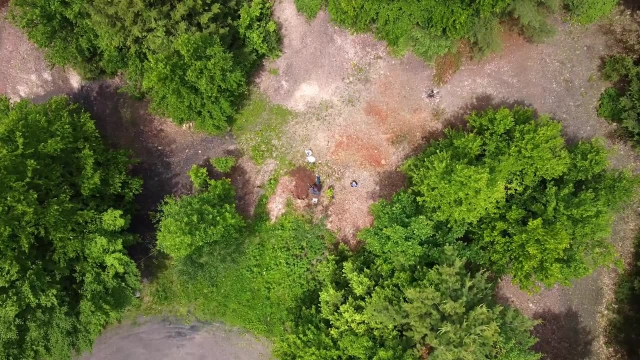 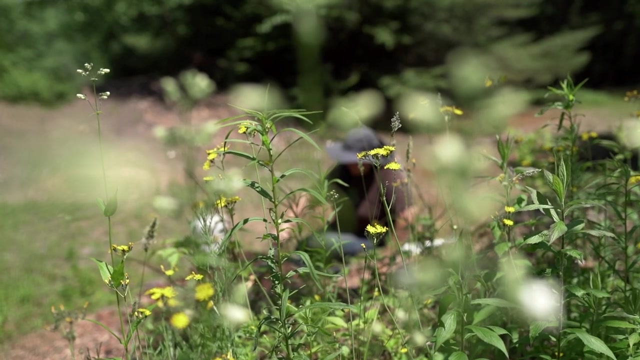 widely circulated pictorial representation of a scene from prehistoric life, based it on fossils, Anning had found and sold prints of it for her benefit. More likely, if there is something in there it will split open, because the fossil had decayed the organic material away and it left a little cavity in there. so that is a weak. 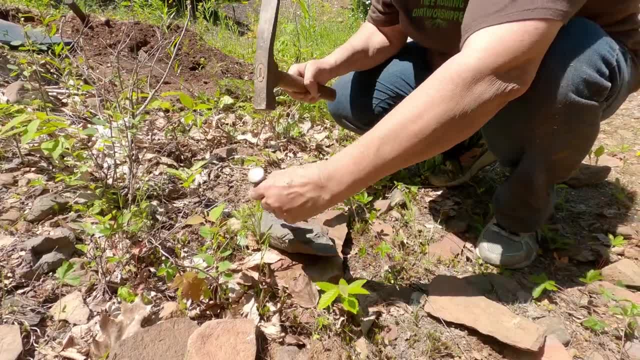 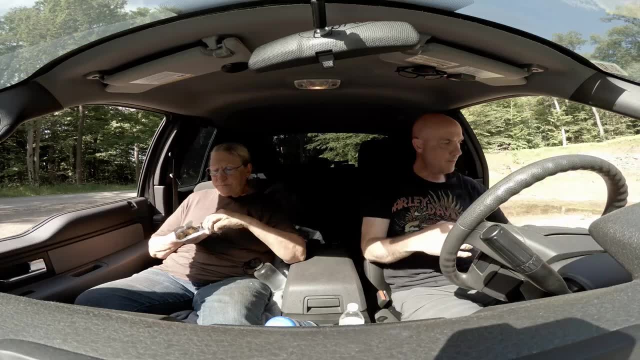 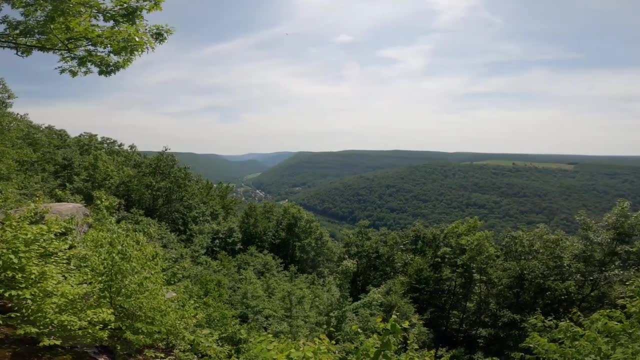 part of the rock. now, As we took a break to have lunch and check out the nearby overlook, my mother and I discussed the differences between paleontologists and archaeologists. I made the statement that paleontologists would never be as cool as archaeologists. I referred to my childhood. 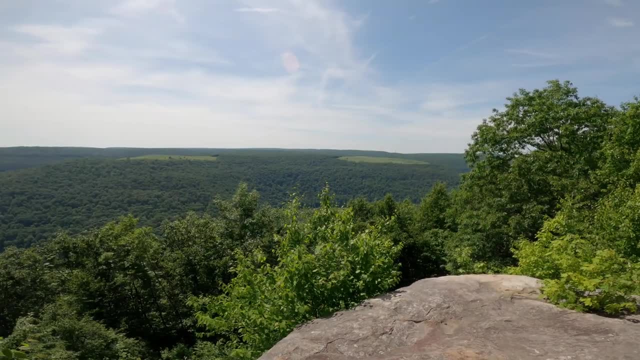 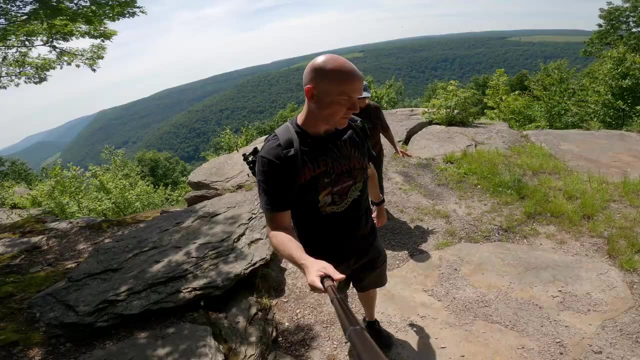 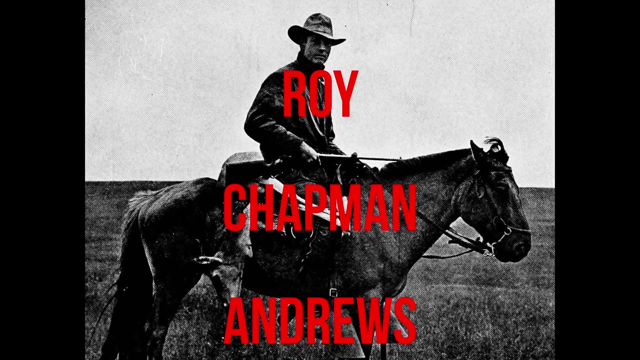 hero fictional archaeologist, Indiana Jones. Our debate eventually forced me to start researching online later that night. Apparently, Indiana Jones' character is believed to be based on a real-life paleontologist: Yeah, Roy Chapman Andrews. Andrews was born in 1884 and died in 1960.. He was an American explorer, adventurer and 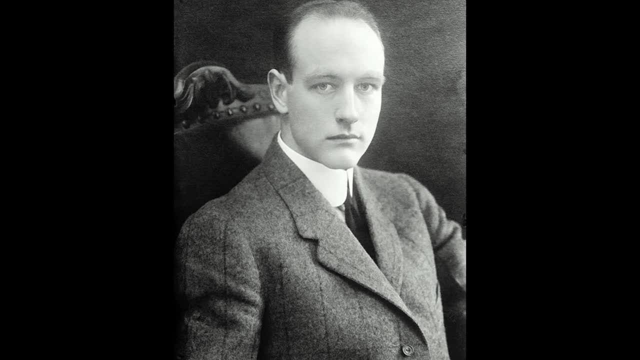 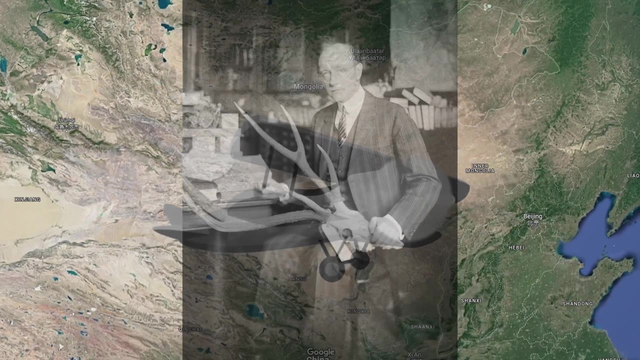 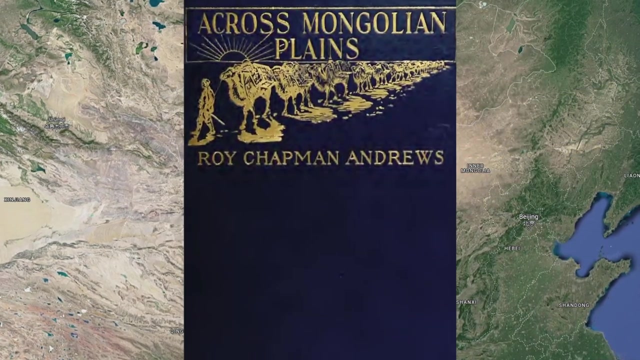 naturalist who became the director of the American Museum of Natural History. He led a series of expeditions through China into the Gobi Desert in Mongolia. Among many other discoveries, these expeditions brought the first known dinosaur eggs to the museum. His popular writing about his adventures made him famous. Andrews joined the Explorers Club. in 1908. The first time Andrews was born was four years after its founding. 1909-1910, Andrews sailed on the USS Albatross to the East Indies. 1913, he sailed aboard the Schooner Adventurers to the Arctic. 1922, he discovered a fossil of a gigantic hornless rhinoceros. The species. 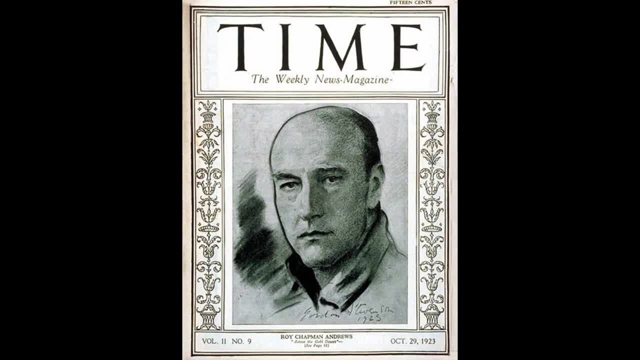 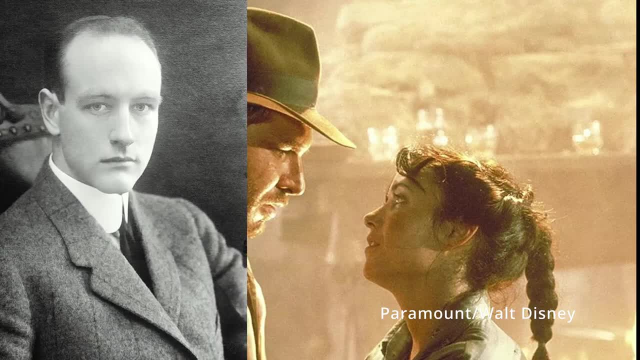 was named after him the first nest full of dinosaur eggs ever discovered 1942,. he retired to North Colebrook, Connecticut, where he wrote most of his books about life and adventures. So apparently paleontologists are pretty cool. So you see that there's…. 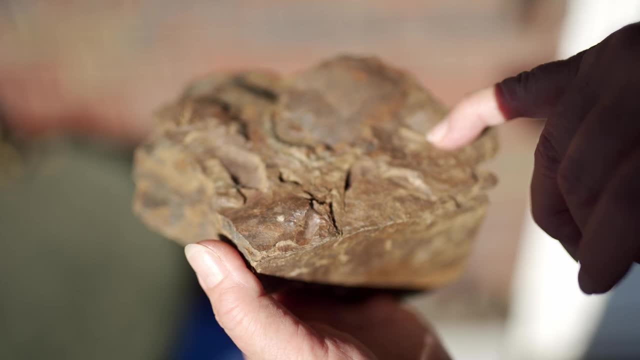 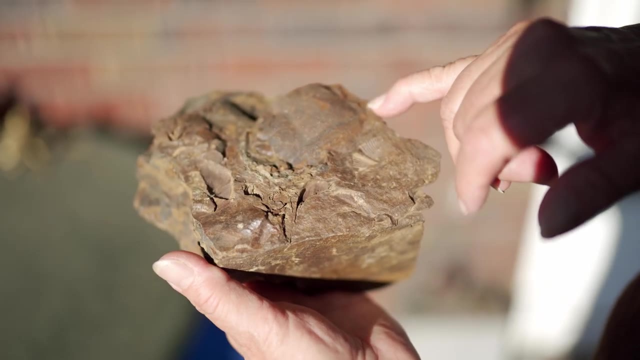 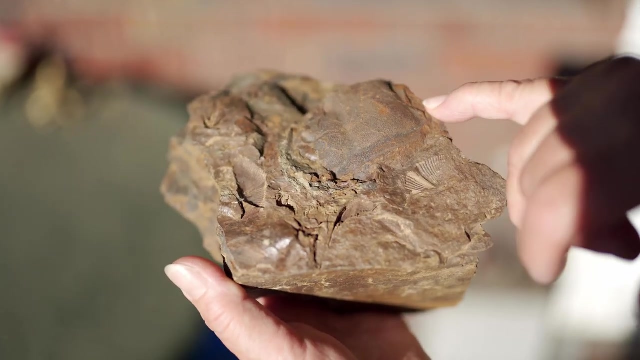 There's. There's a cycle. There's a cycle that there's a lot of marine life in here- shell fossils- but what is really intriguing about this is there's a huge trilobite head here. this is where the eye was on this side and of course, this eye over here is broken off, so you can't.